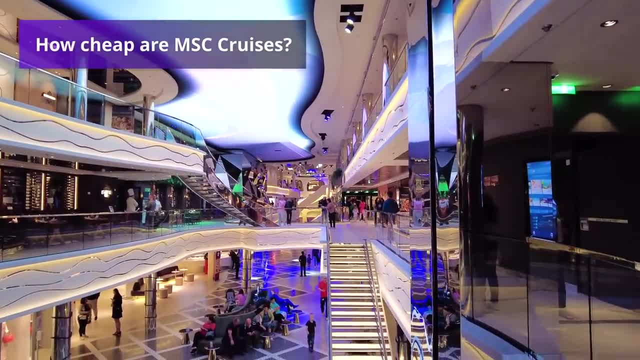 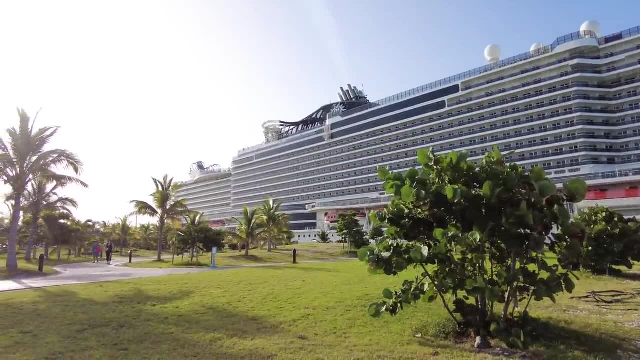 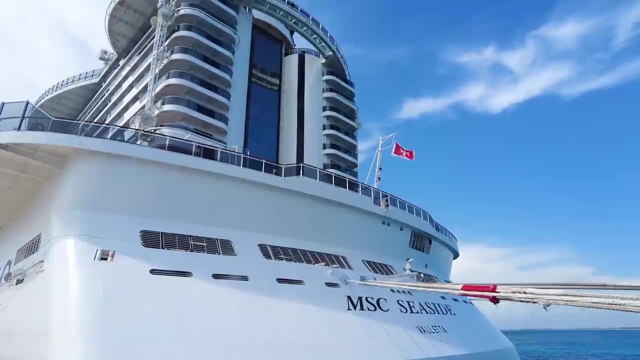 So how cheap are MSC Cruises? MSC Cruises has been growing in popularity, with cruises leaving from several US ports such as Miami, New York, Port Canaveral and Galveston starting in 2025.. A major factor for this growth has been price, and, glancing at their fares, we can see why so many cruisers are giving the cruise line a try. Looking at current MSC Cruise deals, there are some pretty low cruise fares. If you're dreaming of a cruise to the sunny Western Caribbean, MSC has a 7-night sailing for $200 leaving from Port Canaveral on MSC Seaside, including a stop at their popular private island, Ocean Cay. 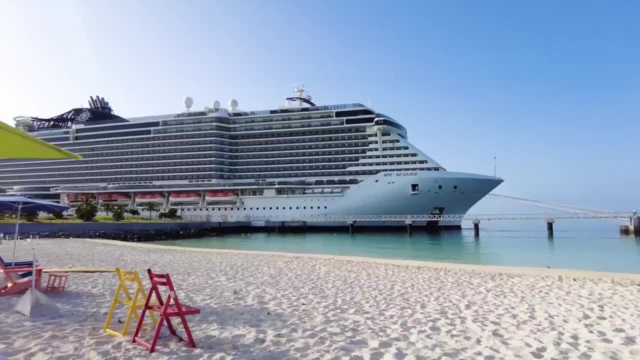 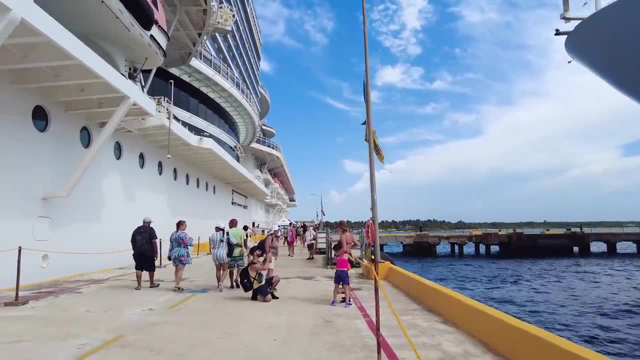 Compare that to MSC Cruises. They set rate to $450 per person on Carnival Magic and $420 per person on the Brilliance of the Seas for week-long cruises in the Caribbean. In terms of the age of the ship, MSC Seaside was launched in 2016,, and it's much newer than Brilliance of the Seas. 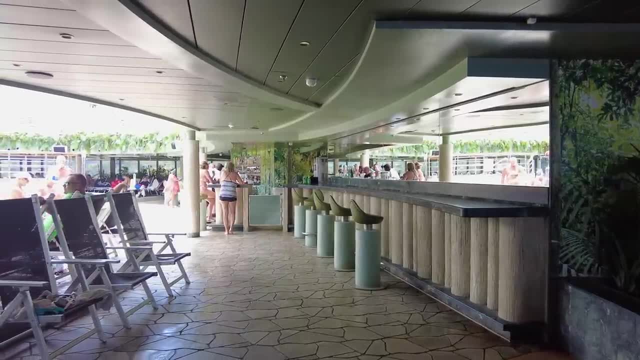 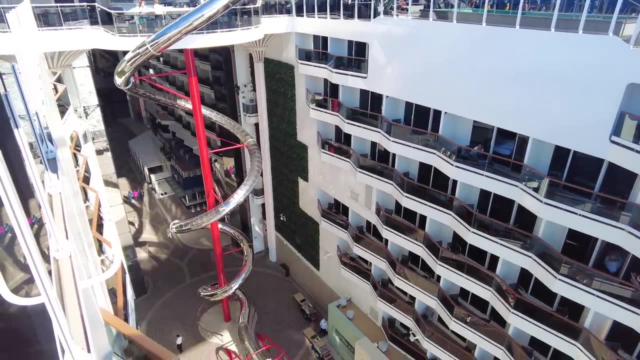 which set sail in 2001, and Carnival Magic in 2010.. How is MSC Cruises able to offer such low prices? They have some financial strategies to help manage profitability While embarking on these aggressive marketing strategies to grow market share. Strategy number one is cost control. MSC stretches their passenger-to-crew ratio to keep costs down. One of the biggest expense categories for cruise ships is payroll costs. Carnival, one of MSC Cruises' main competitors, notes on its financial statements that labor costs are their single largest expense, at 18% of total revenues. That's a little over $2 billion in payroll costs. Being able to effectively manage these costs can translate to significant savings on the bottom line. Cruise lines like MSC need to watch these costs closely if they want to lead the market on price. One of the ways MSC Cruises can manage these costs is by stretching the passenger-to-crew ratio. 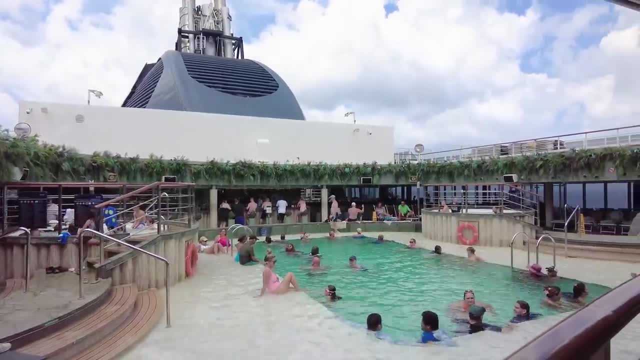 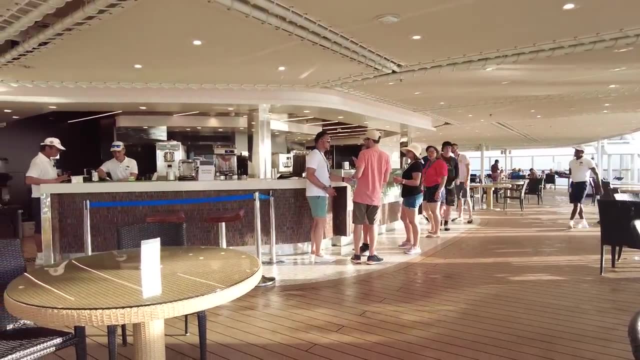 In simple terms, this is the number of passengers divided by the total number of crew. The higher the ratio, the more people a crew member needs to attend to, which can impact service levels. To get a sense of the average number of passengers, there are specific protocols required. of these ratios. I looked at some newer ships. among the mass market cruise lines, The best ratio was Norwegian Prima at 1.99,, followed by Royal Caribbean's Wonder of the Seas at 2.4,, MSC Seascape at 2.75, and Carnival Celebration at 3.04.. MSC's ratio is one of the highest. 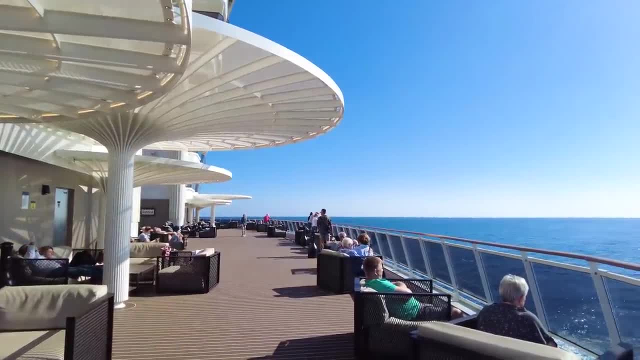 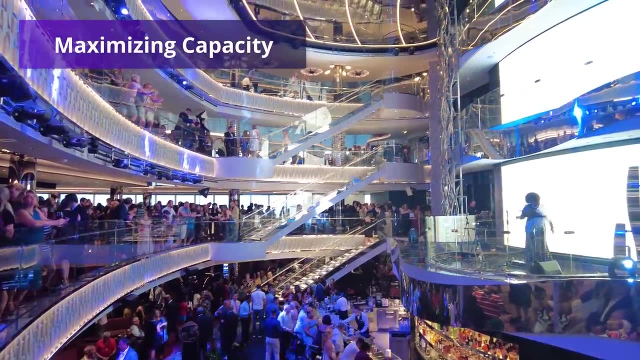 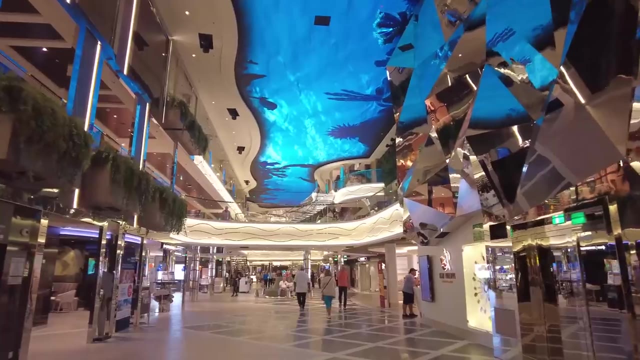 although lower than Carnival. One of the ways that MSC can offer cheap cruises is by maximizing the number of guests it welcomes on board. While management of crew costs is one part of the financial equation, maximizing revenue is another. How do cruise lines do this? They get as many. 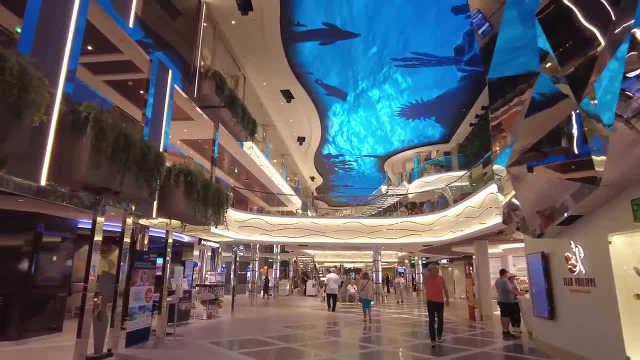 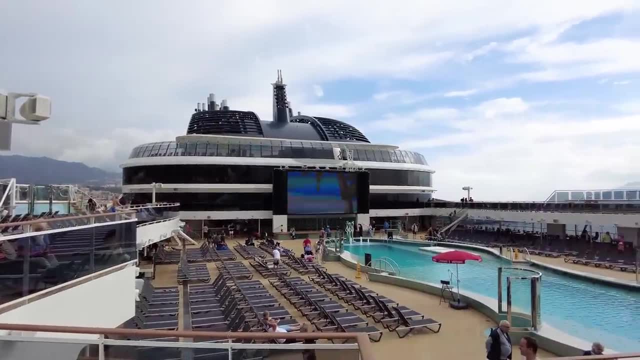 passengers as they can on board. This is especially important as cruise lines charge per person and not per cabin. Similar to the passenger-crew ratio, a space ratio helps us to compare cruise lines and how effectively they use their space to maximize earnings. A common measurement used in cruise. 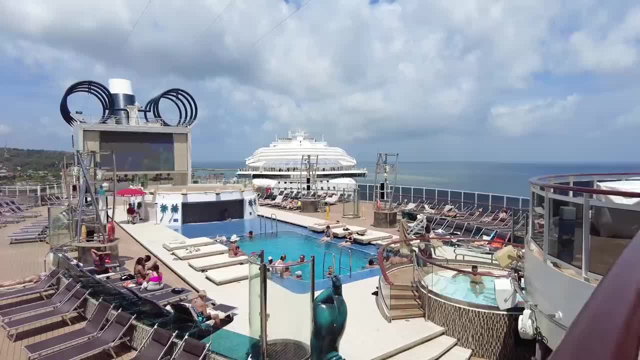 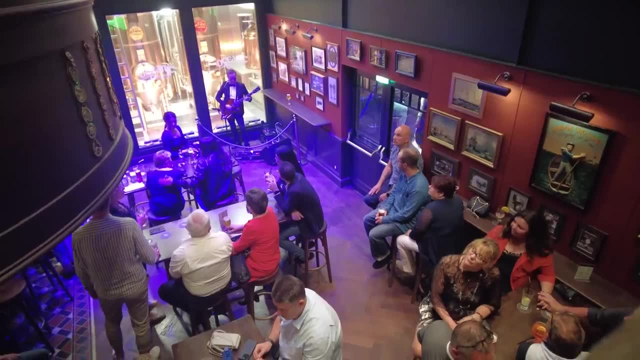 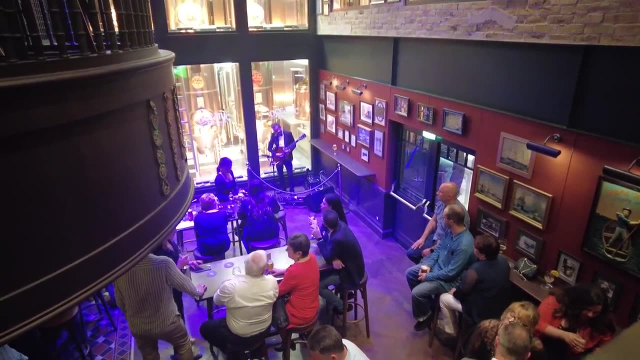 lines is gross tonnage, Which is a measure of the inside volume of the ship. Gross tonnage divided by passenger numbers gives a comparable space ratio. when evaluating different cruise lines, I looked at the same cruise ships as before and, not surprisingly, they ranked in the same order as their service ratios. 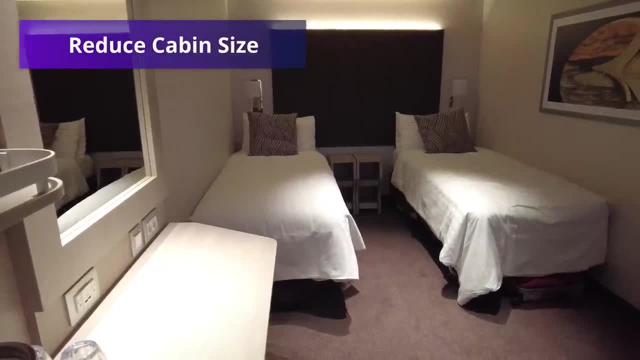 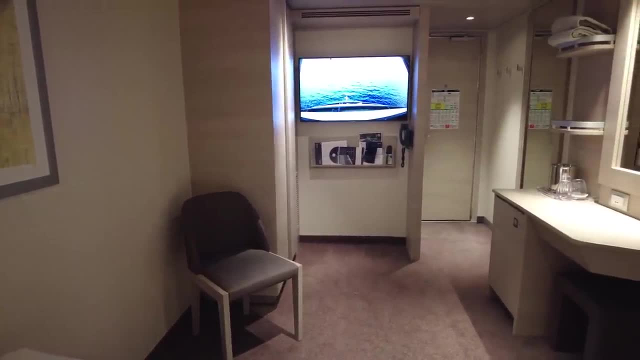 Another strategy is that MSC reduces cabin size to save money. Every passenger needs a place to lay their head somewhere at night. Cruise lines like MSC who want to achieve optimal passenger count have a space ratio of 1.99.. MSC's ratio is 1.99.. MSC's ratio is 1.99.. MSC's ratio is 1.99. 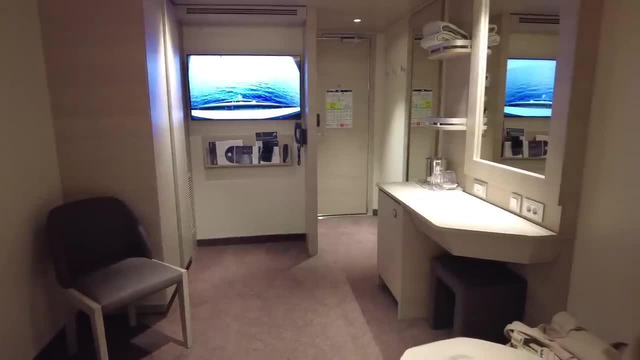 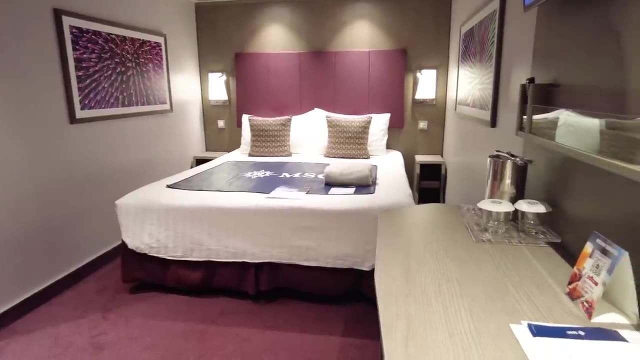 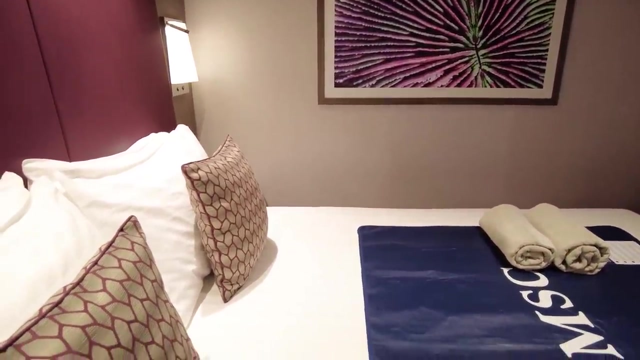 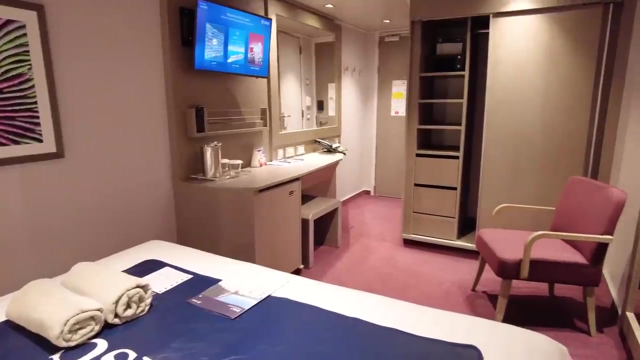 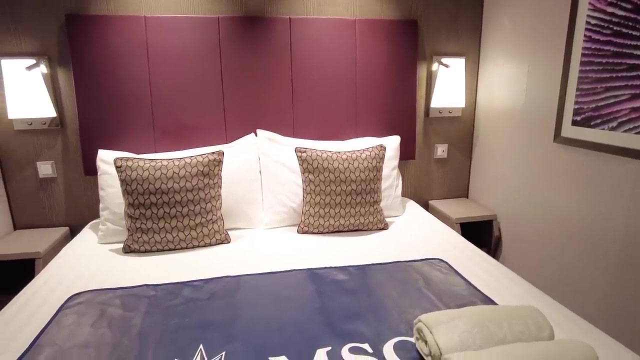 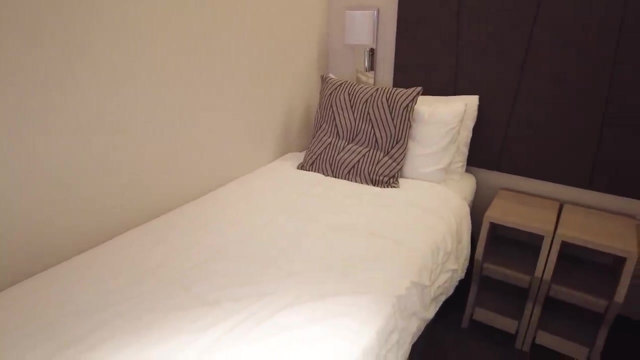 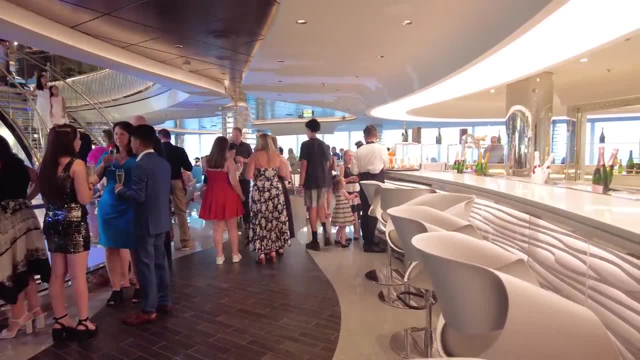 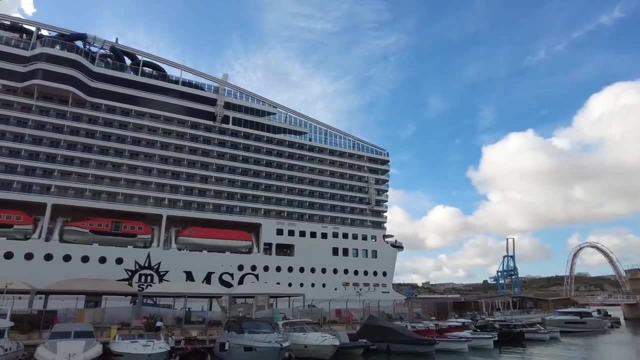 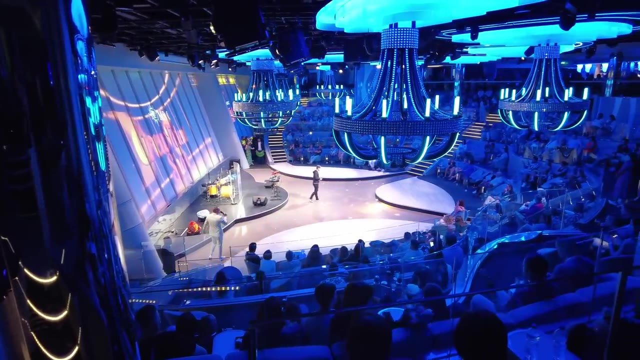 MSC Cruises is part of the larger MSC Group, a shipping conglomerate with sizable assets. The company is privately held, but some analysts estimate the shipping empire to be worth $100 billion thanks to their diversified holdings in shipping cruises, cargo ferries and more. 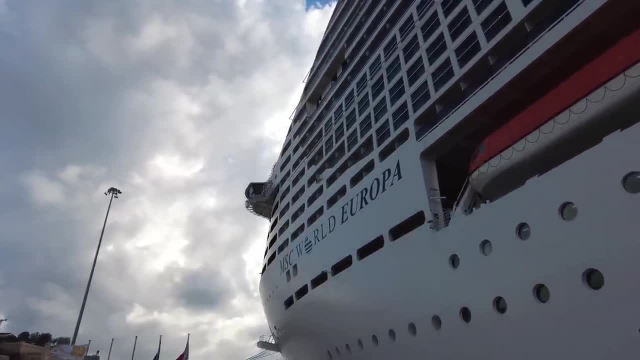 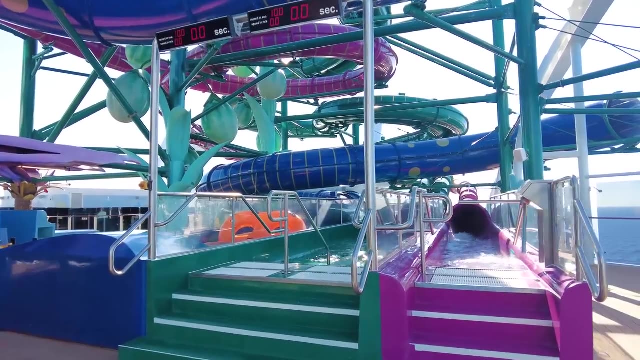 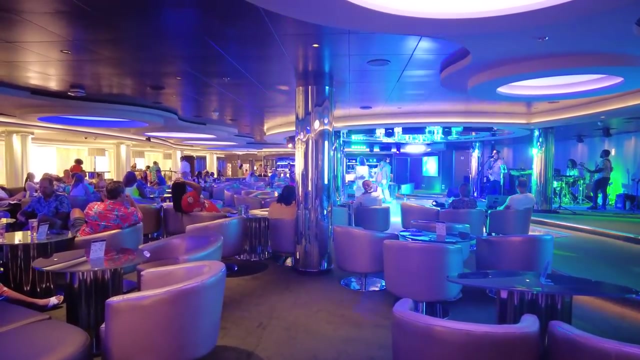 Large companies with deep pockets, like MSC, can implement short-term strategies to gain market with lower prices. Also, because MSC is privately held, they don't need to focus as much on short-term earnings, but rather on long-term profitability, with no dividends for shareholders to worry about. 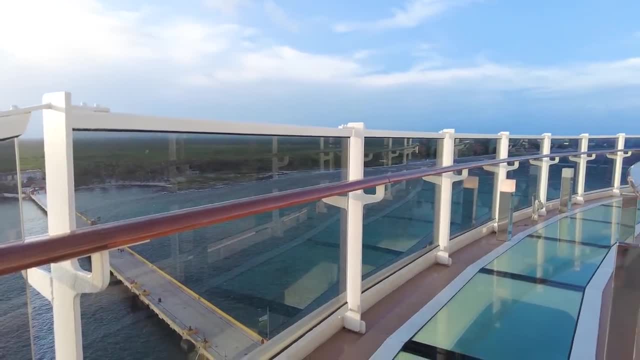 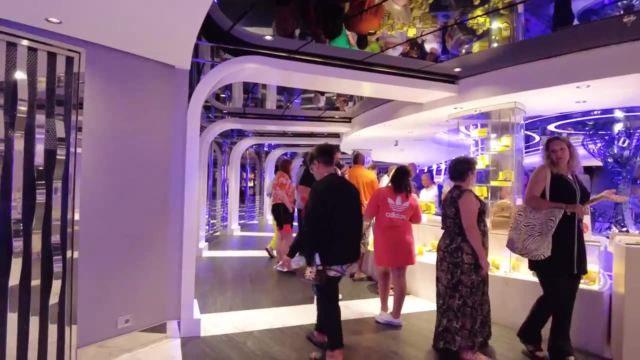 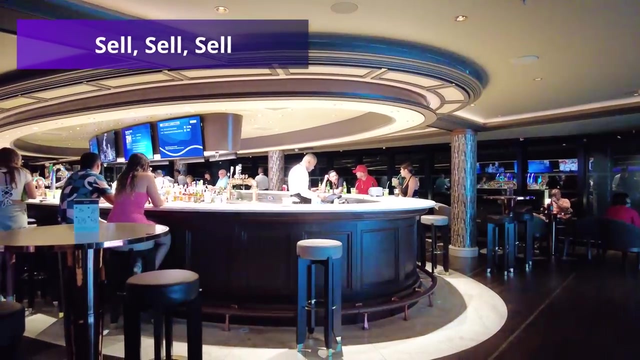 While it's not known what their debt and equity structure is. like a private company can. They can reinvest funds and sell finance expansion along with private funding options. Their next strategy is sell, sell, sell. MSC Cruises upsells numerous onboard services and add-ons. Everything from drink packages to Wi-Fi excursions, specialty dining spas and even entertainment like bowling and race car simulators. These extras really add up. On MSC ships, activities like racing are $12 per person and movies are $11,, which can quickly add up. Most of their add-on packages are cheaper if booked pre-cruise, enticing customers to lock in savings, and the cruise line provides lots of options. Guests can choose from five different drink packages, eight different Wi-Fi packages and several specialty dining combinations. 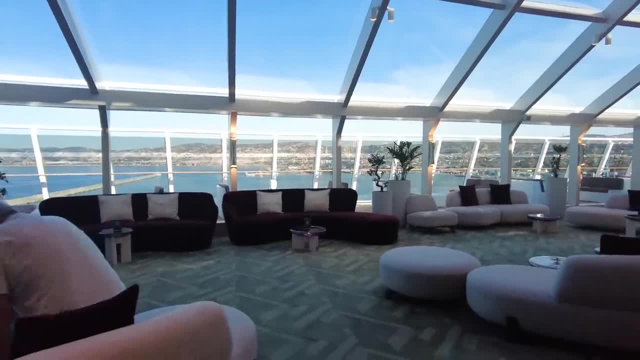 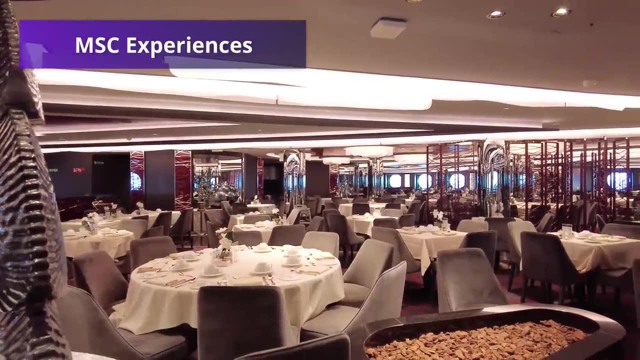 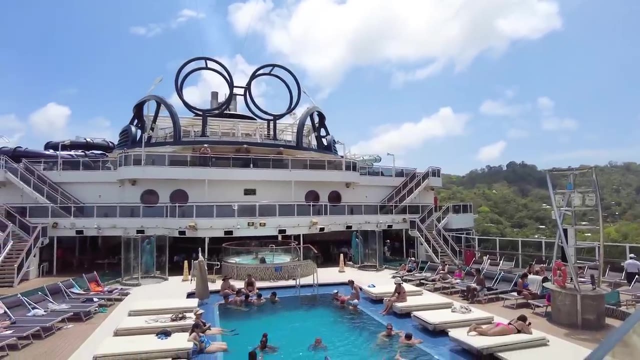 providing something for every budget and preference. Another strategy of MSC is the MSC Experiences. They provide additional revenue for the cruise line. something unique when booking an MSC cruise is that guests can select from five distinct MSC Experiences in addition to their cabin options. 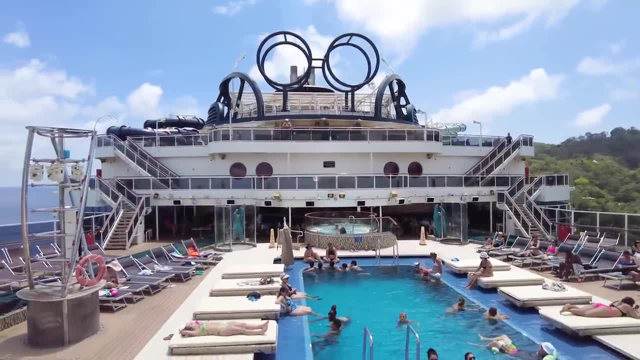 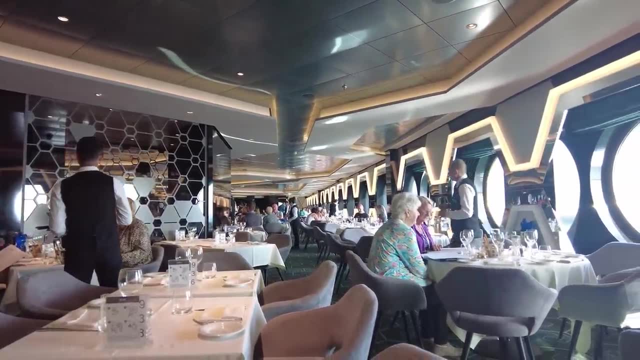 The lowest tier. Bella has the best value prices, but also has bare-bone perks compared to upgraded Experiences like Fantastica and Aurea, For example, Bella cabins include the basics, such as food, entertainment and cabin attendant service. 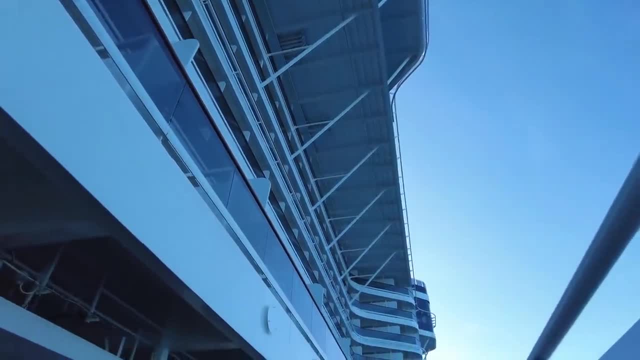 However, if cruisers upgrade to Fantastica, they get one free cruise ticket and they can also get a free ticket to the MSC cruise. However, if cruisers upgrade to Fantastica, they get one free ticket to the MSC cruise. 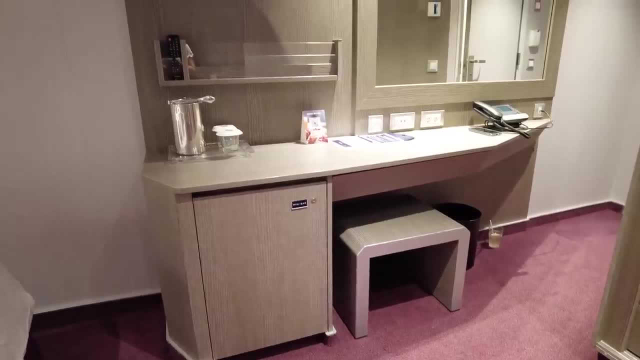 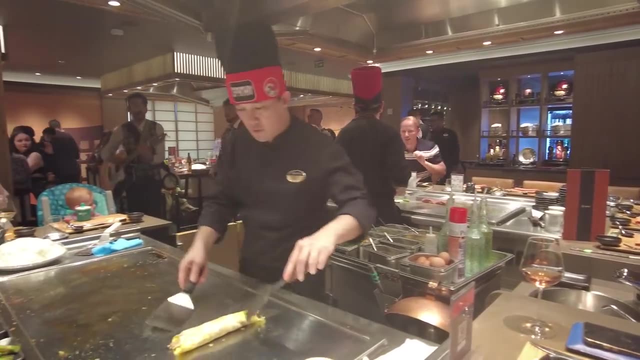 and they can also get a free ticket to the MSC cruise. However, if cruisers upgrade to Fantastica, free breakfast delivery in their cabin, the ability to choose their room location, 20% off specialty dining packages and the ability to request their preferred dining time. For a seven-night cruise to the Caribbean. the upgrade is currently priced at $140 per person. As guests move up to Aurea, the benefits become even more, and so too are the prices. MSC allows its guests to customize the cruise experience. 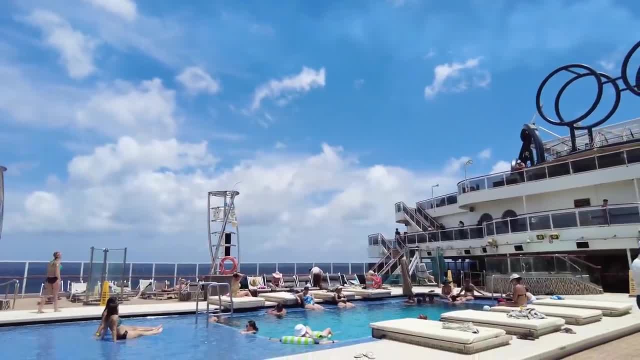 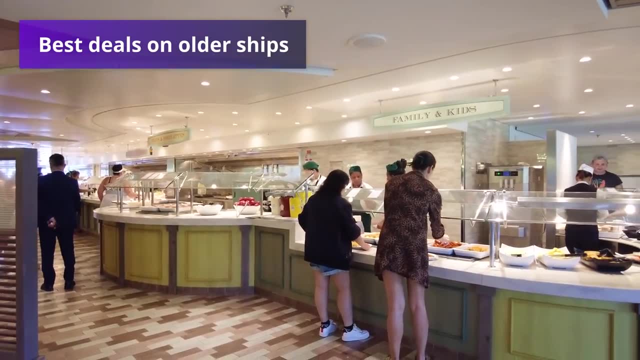 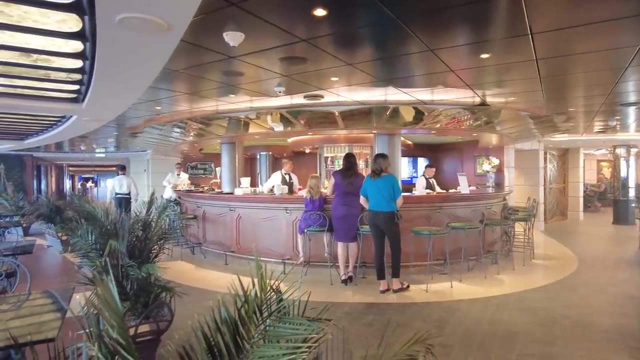 but the super cheap cruise prices offer the basic cruise experience. The last strategy is that many of MSC's best deals are on older ships. While MSC Cruises has been on a building spree, having launched eight ships in the last five years, there are still many older ships in the fleet, In fact, 12 of their ships. 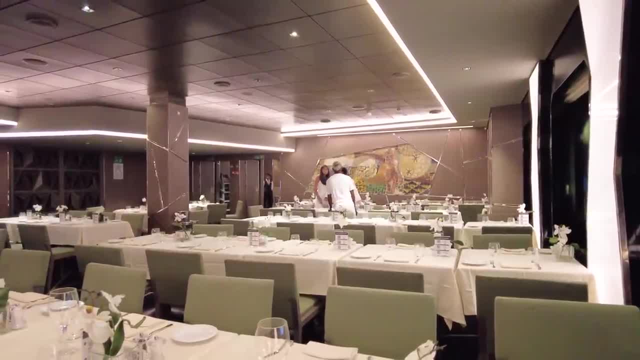 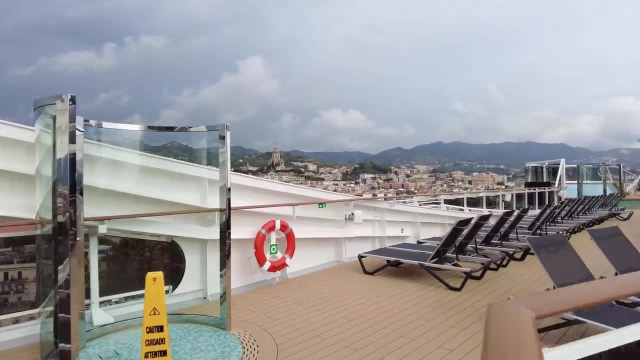 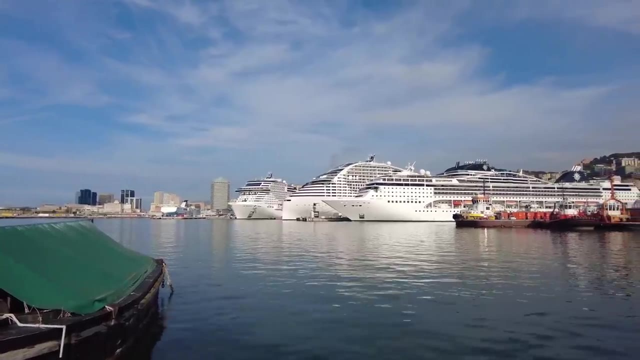 are at least 10 years old, with the oldest being MSC Harmonia, which was launched in the year 2000.. MSC Cruises has an incredibly strong presence in the European cruise market, offering tons of cruises at bargain prices with ships like MSC Fantasia, MSC Lyrica and MSC Poesia, While the 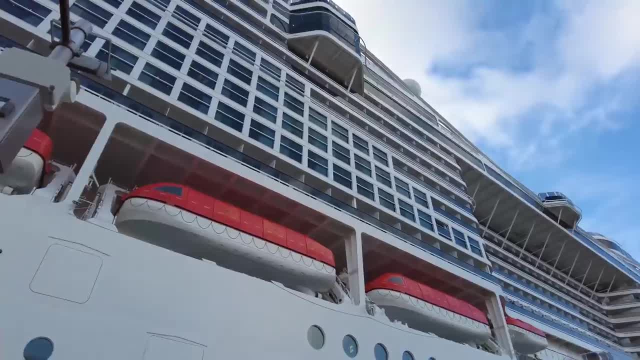 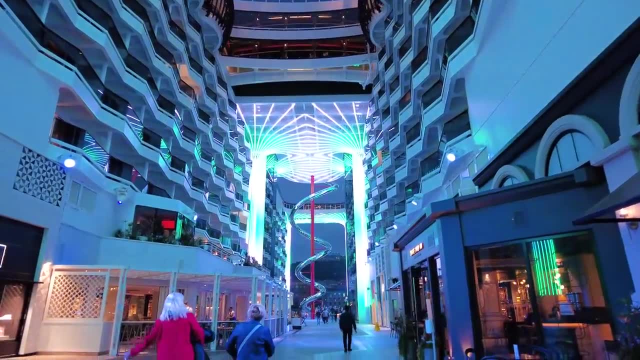 ships offer the classic cruise experience. they may not have all the bells and whistles of the new ships, like water parks, slides and other fun activities. So what do cheap cruise fares mean for the MSC Cruise Experience? You still get the basics like food, entertainment and cabin. 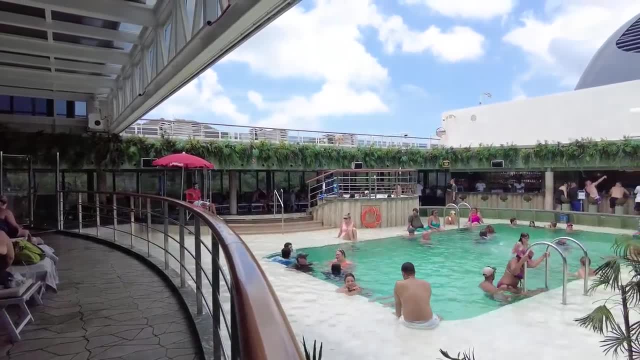 options. but these low prices come with limited perks. Also, there's a lot of fun in the MSC Cruise Experience. and there's a lot of fun in the MSC Cruise Experience. There are many upgrades and packages you can purchase which can quickly add up. 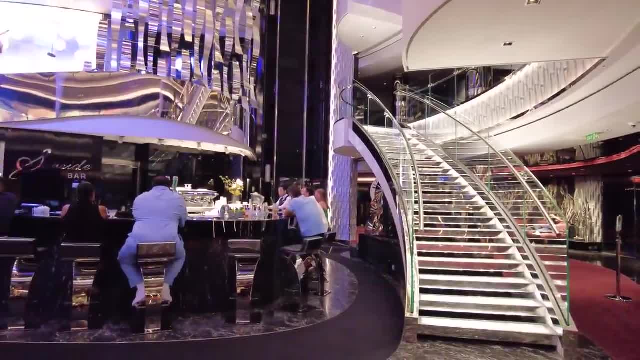 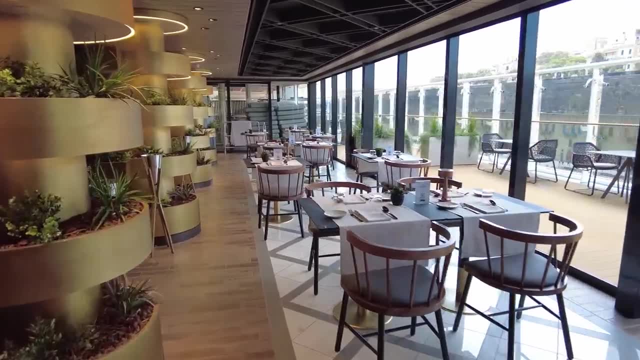 I have enjoyed my MSC Cruise Experiences, but having the right expectations and knowing what's not included is important. In particular, their newer ships are beautifully designed and have lots of light and space. I found the MSC Seascape to be as nice as Celebrity Edge.